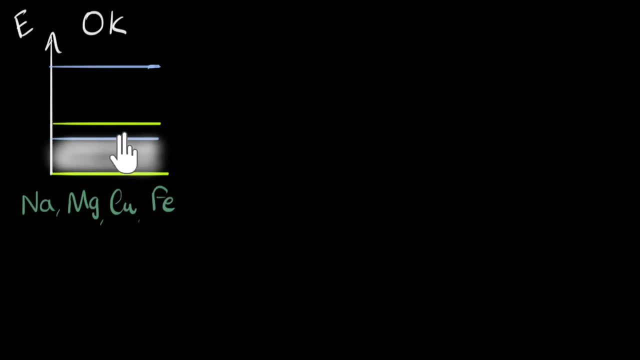 energy band. So I really should get rid of these divisions over here. I'm just going to decrease their opacity. There you go. So what we have now is one giant energy band with electrons not completely filled. There are so many vacant spaces at zero, Kelvin. Now think about what will. 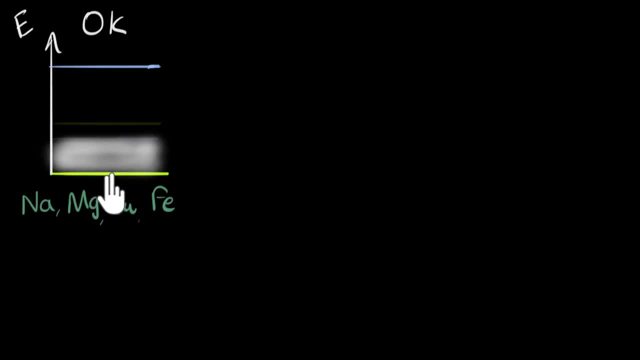 happen if we increase the temperature just a little bit. If we increase the temperature just a little bit, the thermal energy is going to try and excite the electrons- electrons over here a little bit higher. The question is: are there energies allowed a little bit? 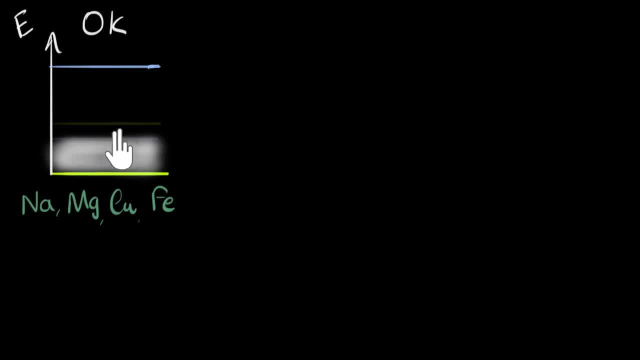 higher. The answer is yes, there are energies allowed. There are so many energies allowed. This is the whole thing, is a continuum. remember, You don't have to jump anywhere over here, It's allowed. And so, as a result, all these electrons, all of them, end up becoming free. 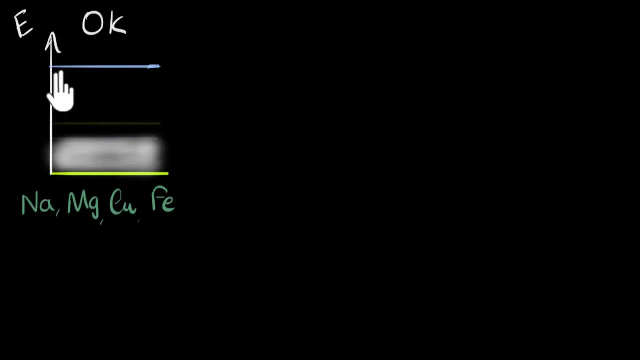 electrons because they can freely move over here. You can sort of think of this like a big classroom which only partially occupied students. The classroom is empty and the kids are going to move around. This is the situation for conductors. So what we're dealing with over here are conductors. 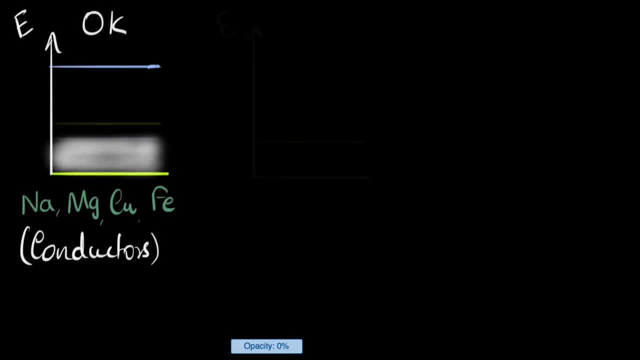 On the other hand, if you look at some other material and check their energy bands, we'll see that their highest energy band- again this is the highest energy band- will be completely filled at zero Kelvin, Will be completely, completely filled at zero Kelvin. 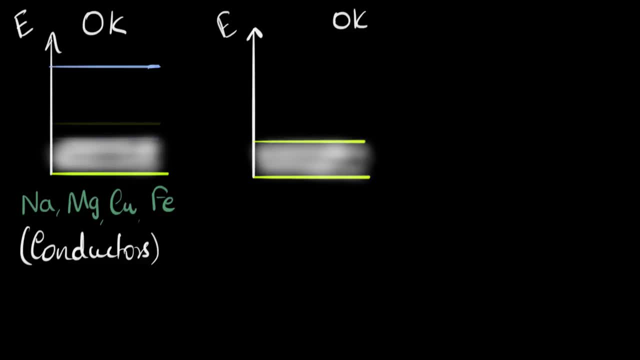 Again, remember, this is okay: zero Kelvin. And now, if you look at their next available energy band, you will see it's not only not it's not overlapping, but there's a huge gap between them. There's a huge energy gap between them. 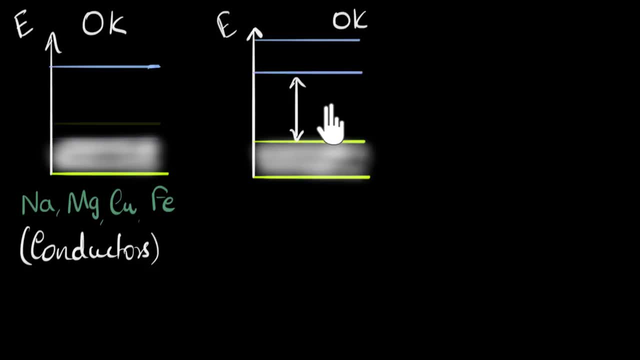 And this energy gap is called as the band gap. It's also called as the forbidden energy levels, because electrons are forbidden to be anywhere over here. Usually we call it as EG. And if this band gap, EG, if it is somewhat more than four electron volt, 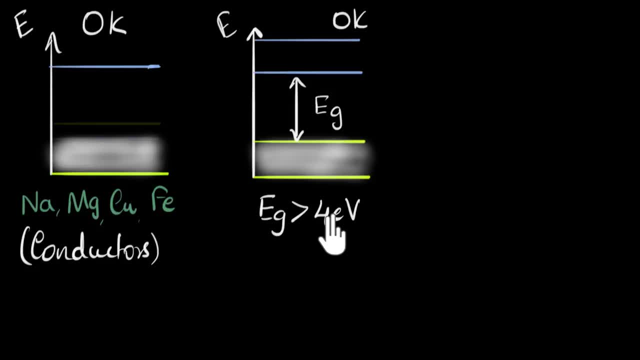 now it's not again. this is not a very strict thing. Sometimes you can write five electron volts or four, but if it's sort of like more than four electron volts, then we'll call this as an insulator. We'll call this as insulators. 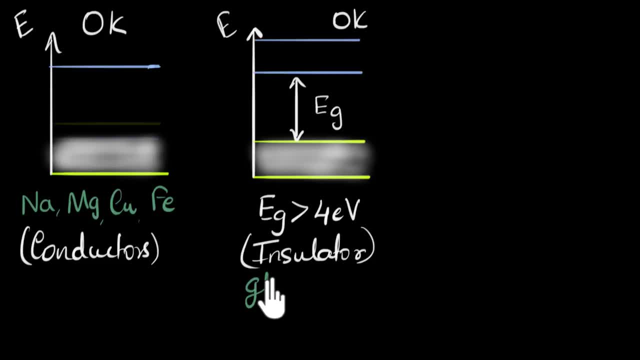 All right. So this will be the example for, say, glass or diamond. They're excellent insulators. Can you see why they end up becoming insulators? Because now, if you increase the temperature a little bit, and the electrons tried to get excited. well, now the electrons can't get excited so easily. 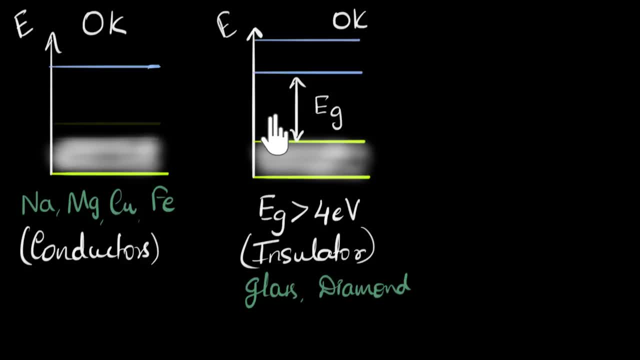 because if you try to excite the electron from here to here, well, they can't accept that because, remember, these energy levels are forbidden. So if you want to excite these electrons, you have to excite them all the way till here. 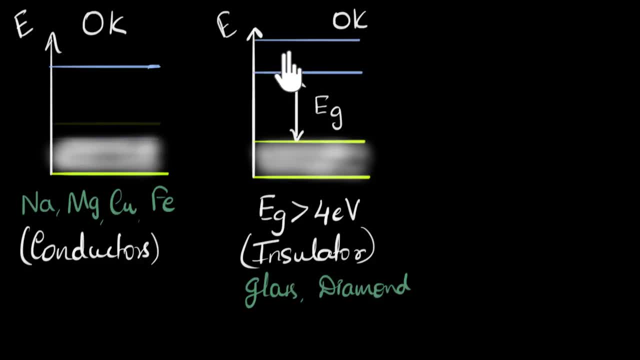 And the probability of an electron being excited all the way over there is extremely low, even at room temperatures, And so in such materials, even at room temperatures, you'll find extremely tiny amount of electrons found in this empty band, and so only little bit of. 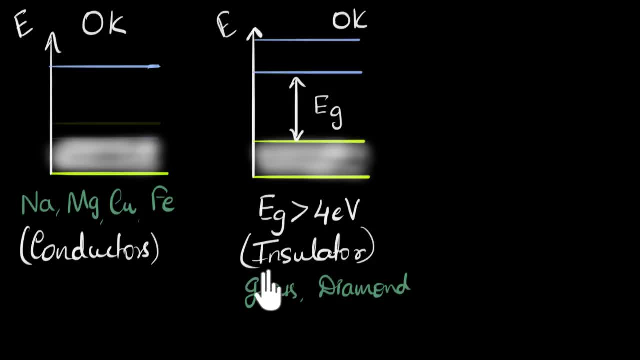 or negligible amount of free electrons are found, And that's the reason insulators behave like insulators. And if you look at silicon or germanium and focus on their highest energy bands, again it's found that at zero kelvin. 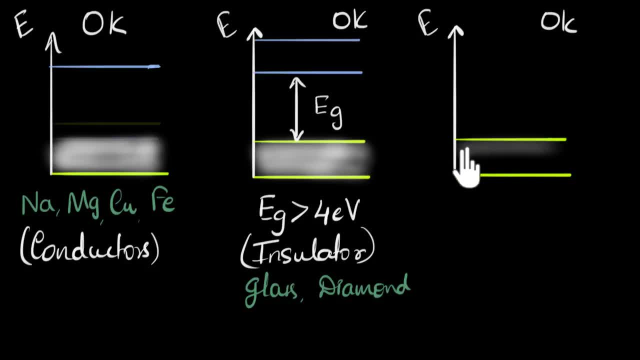 this is completely filled, Zero kelvin. this whole thing is completely filled, just like an insulator. all right, But now, if you look at its next available energy band, what you find? its situation is very similar to insulator. 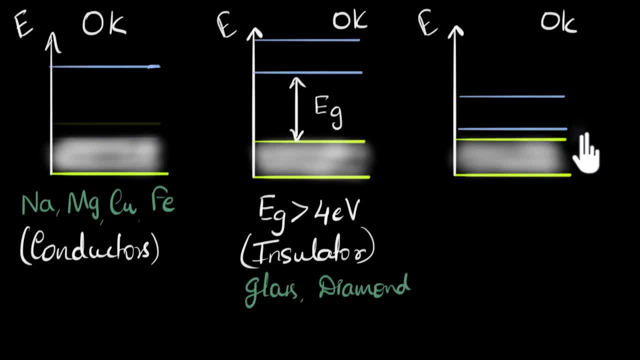 but you can see, the difference is that that same band gap, that forbidden energy gap, that band gap is extremely tiny. Usually it's for silicon. I remember it's for silicon. it's about 1.1 electron volt. 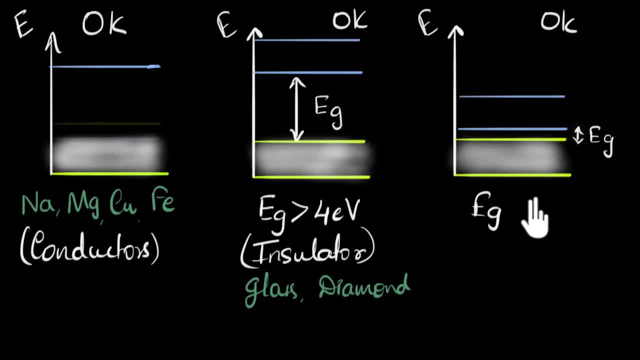 for germanium about .7 electron volt, so it's usually found to be less than about two electron volt. we can say Something like that. Again, it's not very rigorous, we don't have to worry too much. All that matters is very low. 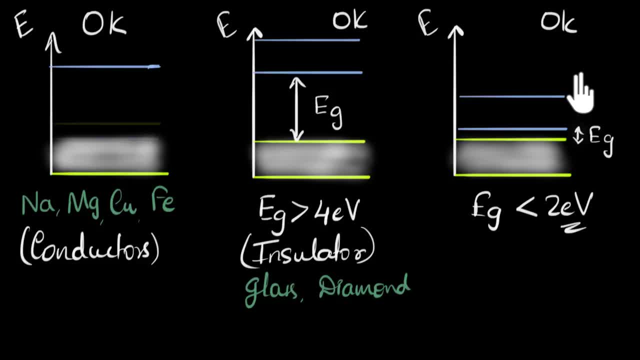 And now, as a result, if you increase the temperature, say to room temperature, and you try to excite the electrons, well, compared to insulators, electrons will get more readily excited over here. So at room temperature you will find a lot more electrons. 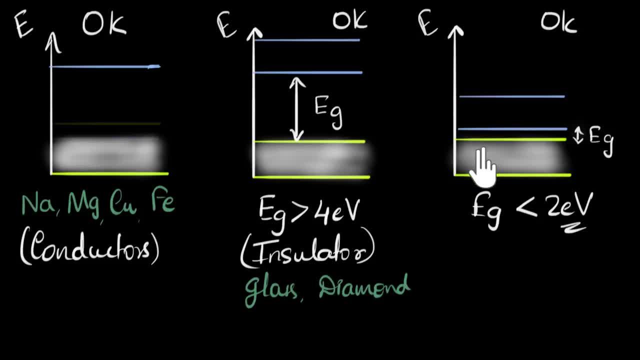 in this higher energy band ready to conduct, compared to that of insulators. But of course they're not as good as conductors, because in conductors you don't have a gap at all, There is no band gap, and so all the electrons.